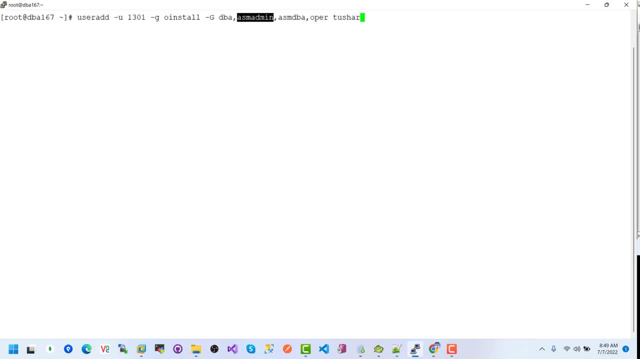 looks here: multiple DBA ASM admin, ASM DBA operator or offer. and this is the username. so after hitting an enter key or user, a Tushar created successfully, so now we need to give the password. as Tushar here, we need to give the password. so I 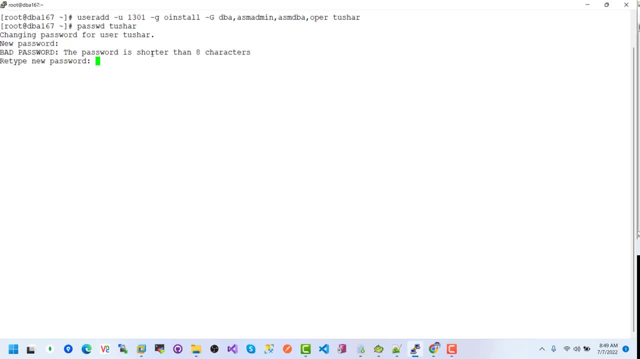 just want to set Tushar so password updated successfully. if you want to give the access or session, as like sys user, to newly created user Tushar, we need to switch the user actually a oracle, so su oracle, and then need to connect with a sql- sql. 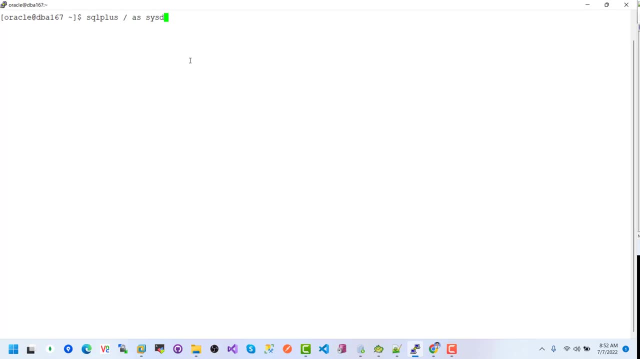 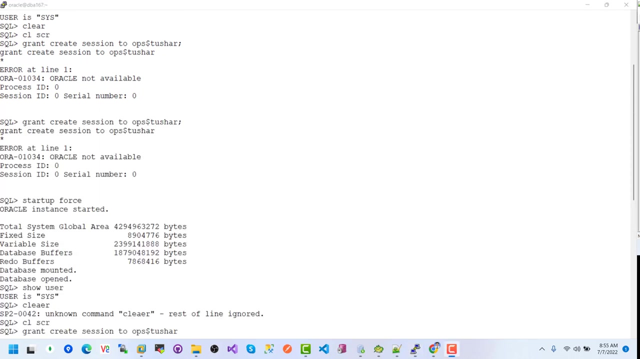 plus slash sys dba. so user- here is sys now output grant and create session to OPS $2 Tushar here. grant oracle. not available grant create session to OPS Tushar here: grant oracle- not available grant. create session to OPS Tushar. when we execute this command: grant create session to ops to serve. this is the username actually. 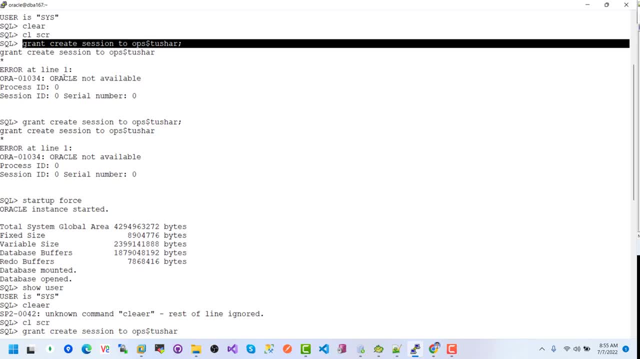 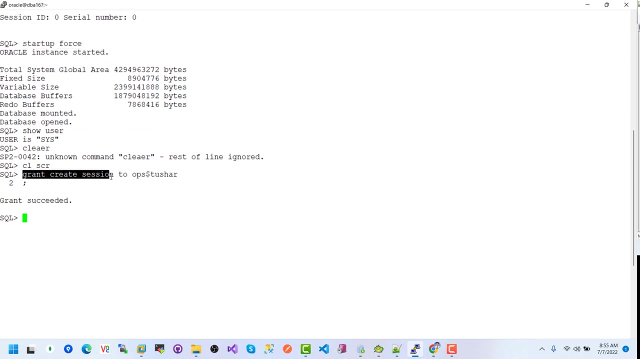 and it's written a error: no, oracle not available. so these types of error we can ignore. if we execute the startup, force means our database instance restarted and after then, if we again execute this command, grant creation to OPS to share grant succeeded. so if I execute this one, 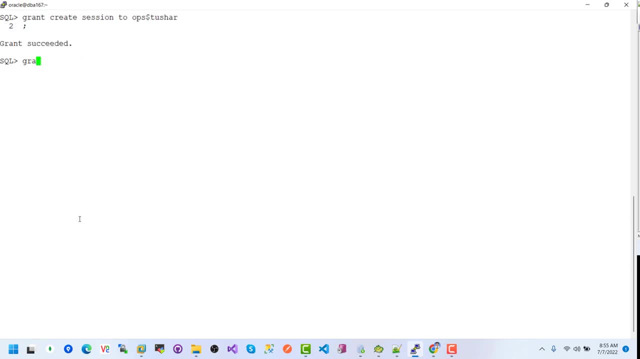 again grant create session to OPS dollar to serve. here we can see the grant succeeded again. now I just want to exit from a square plus here. this is the oracle user, so I just want to switch the user to to serve. yes, to switch user to serve to serve. 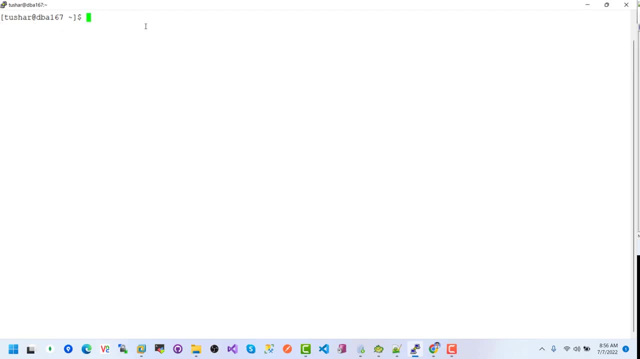 so this is the to serve user. so I just want to connect with sql class. so sql plus slash as sis DBA- here we can see sql plus command not found. so sql flash flash. so here we can see the message command not found. so how do we resolve this issue? let's configure. 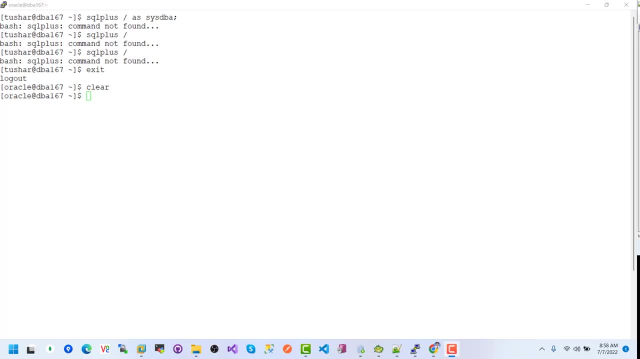 the environment variable, followed by the following commands: let's connect to it uh. switch the user with uh two, uh, two share, two share. so now we need to write here the comment dot, e and v, or uh, dot, dot or a e and v, after hitting an enter key. 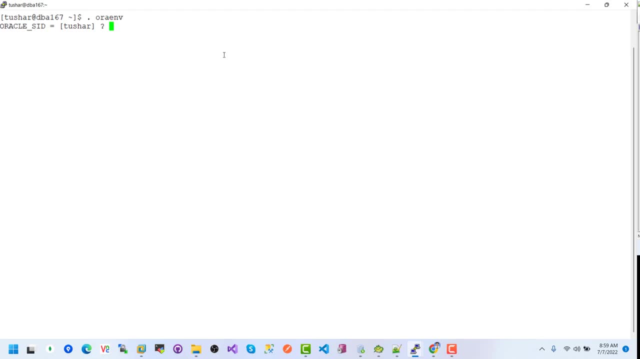 yeah, oracle s ID DBA 167, oracle and bash has been set to here from to this location. let's connect to sql plus, so sql plus slash. here we can see the sql plus connected without any password. so let's connect to sql plus as aata. so let's uncheck it now. okay, so somewhere in sql plus. 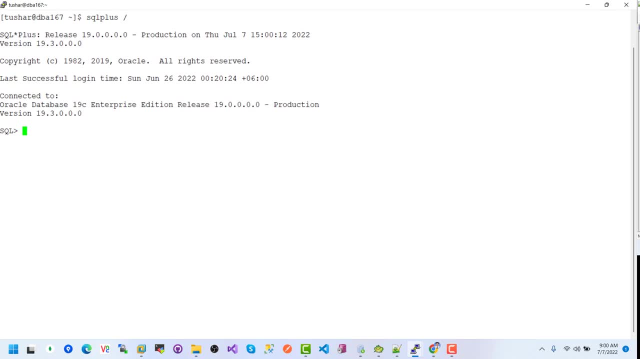 sql fish is connected to sql plus, so this uh two size user is connect with the sql flash more, such as sql uses sql plus side and sql plus name instead ofДitate. no password also had handleれる after transform any tag民 C old user. so in this way we can implement SC assignments located within a username login place. user called magic user. 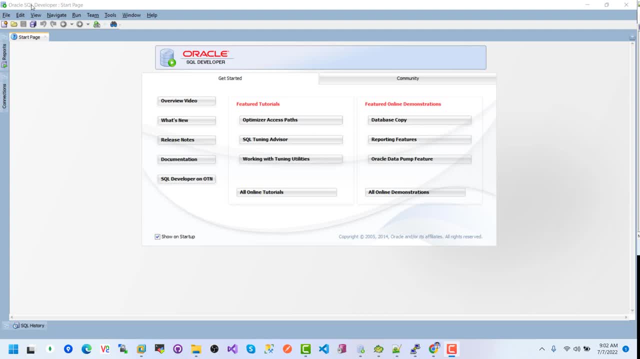 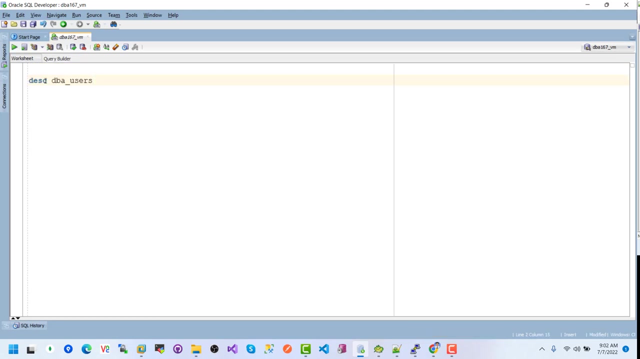 let's check the user status. this is the oracle sql plus developer sql developer actually. so this is the cc user connection, so we need to give the password here. c is one, two, three. okay, this is the worksheet. so here i just want to uh see the email description of dba users. 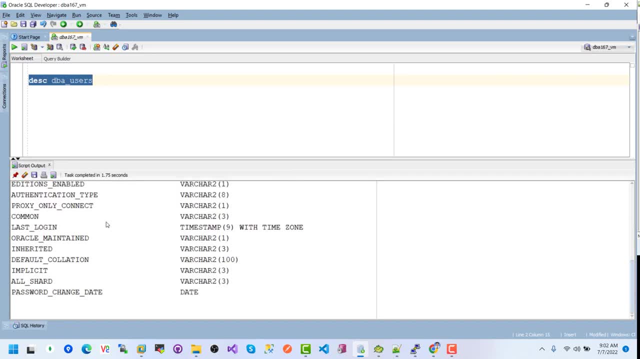 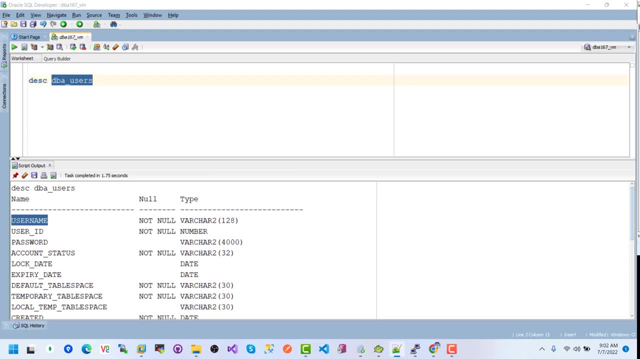 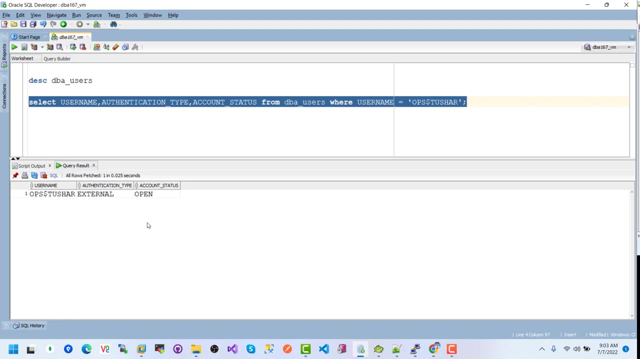 from this description we see the username. so if we execute this command, select username authentication type, then account status from dba user where username is ops to share. so if i execute this one here, we can see this is the authentication type- external and account status open. now look at the password file for cc user. 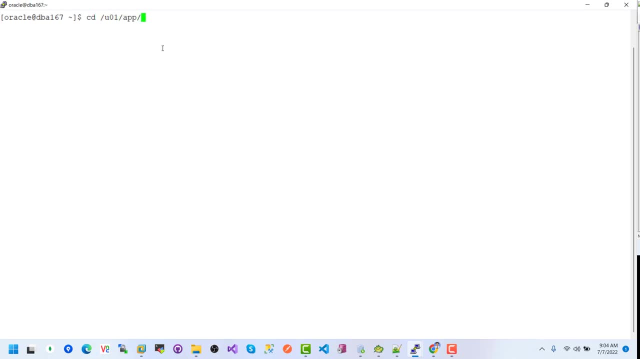 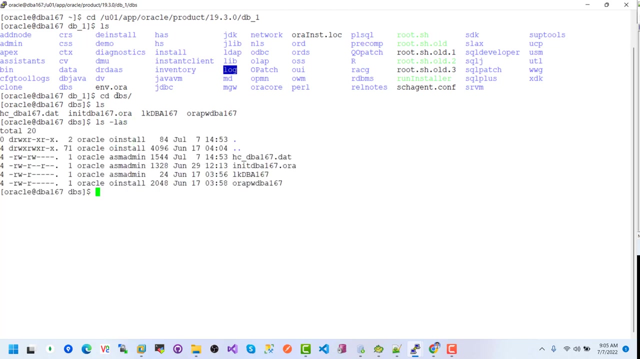 cd slash new zero one slash app. oracle slash product slash 19. c. slash dba underscore one, then db getting an interkey. here we can see the dbs. so cd db s inside this file: location ls minus ls. here we can see the ora pwd db 167. so this is the cc user password credential file. so 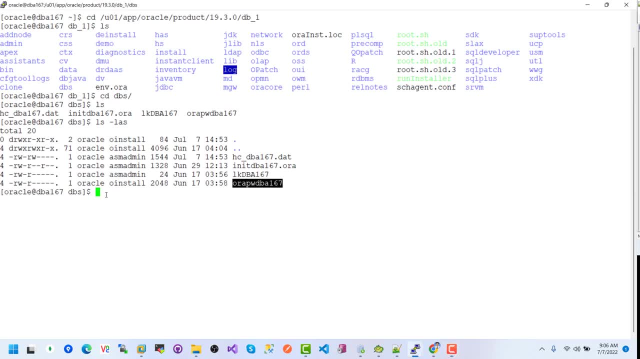 so if we change the file name? so how do we do that? mb, i just want to rename the file name and then new file name underscore. then check the list of file of the file inside this directory. here we can see the password: file name: rename to underscore. so 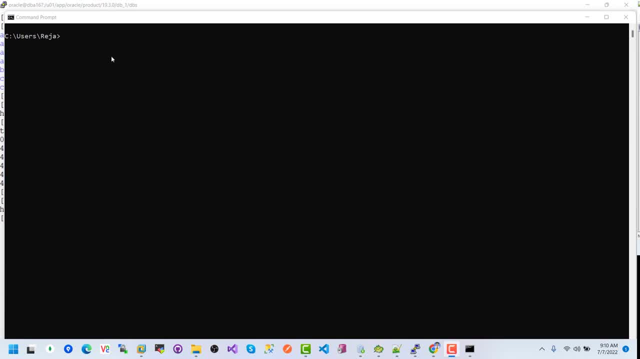 now connect with cc user by client. now connect with cc user by client. so sql plus sql plus slash. so sql plus sql plus slash, c, slash, sys 123, c, slash, sys 123. add at and then add: then this is the dns name, then this is the dns name. 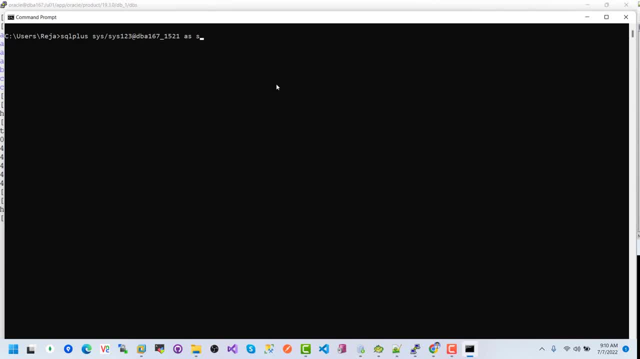 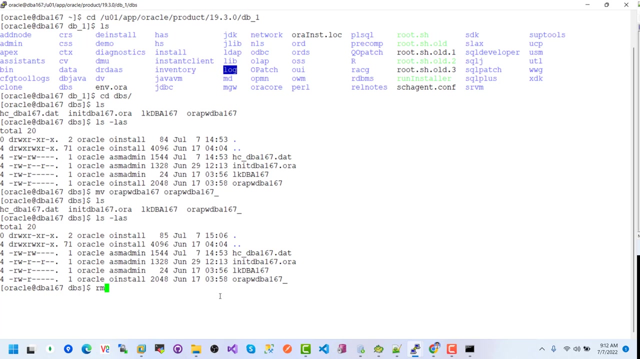 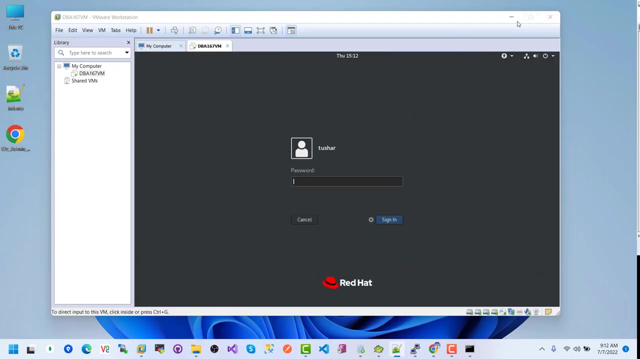 then after hitting on enter key we see the user password not in, not valid, so login denied. now we will rename the file again: MB. this is the modified file and this is the original password file name. so for hitting an enter key for file rename successful: LAS, here we can see this is the password file. so if we try to log in with 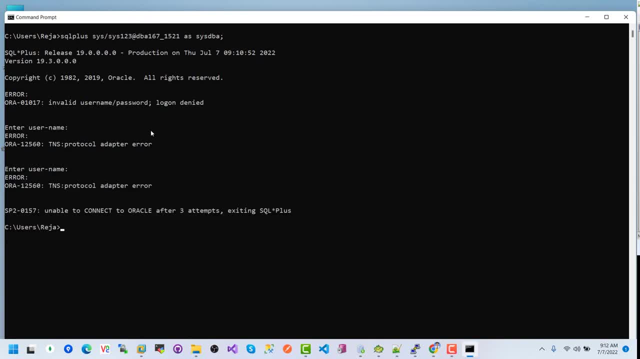 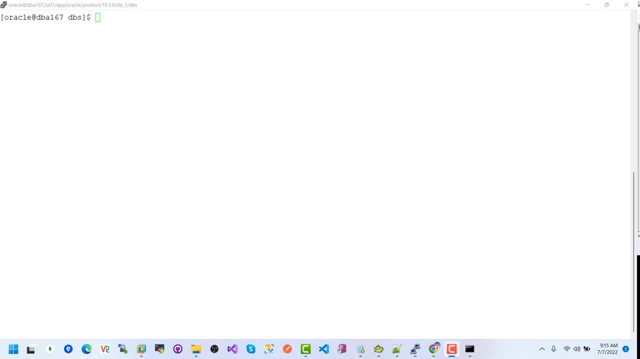 client. so this is our client. so if we try by using this client here, we can see the user CC's are connected successfully. now for the user here- user is 6- creating a user with default profile like a password expiration. so how do you do that? just you need to connect with that spell plus. 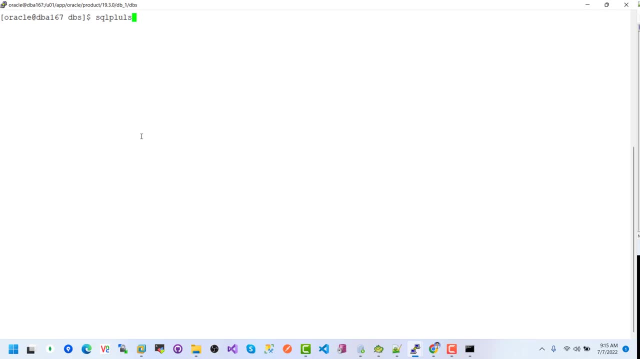 spell class finish and is dbl. userusses is here: clscr. and now we will create a new user. so this is the new user create option by the default profile. so this is the default profile create user. this is the username db167 identified by. this is the password: db167. underscore one, two, three, four default table space users temporary. 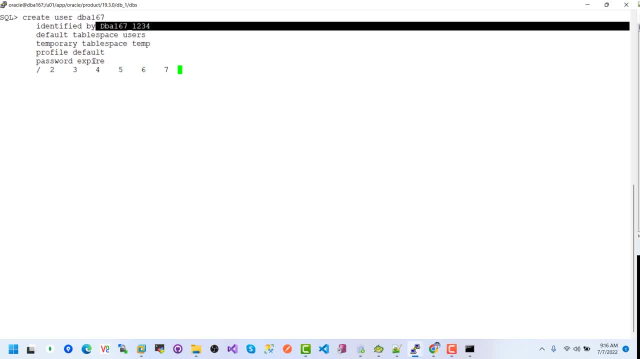 table is streamed, profile default and password expire. so after hitting an enter key here we can see: uh. user db167 conflicts with another user or role name, so first we need to delete this one. so if we execute this one, drop user db167 cascade or user drop successfully. so if i execute this, uh. 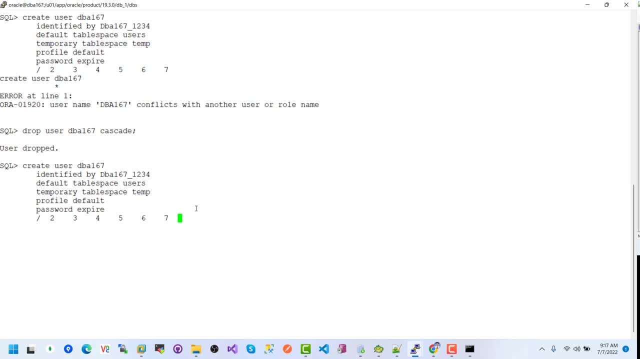 previous command, create user db167. so after hitting an enter key we can see the user created successfully. so now we need to give the creation privilege. so grant creation to db167. grant successful and after then it will ask to change the password from user profile settings, default user profile settings actually. so 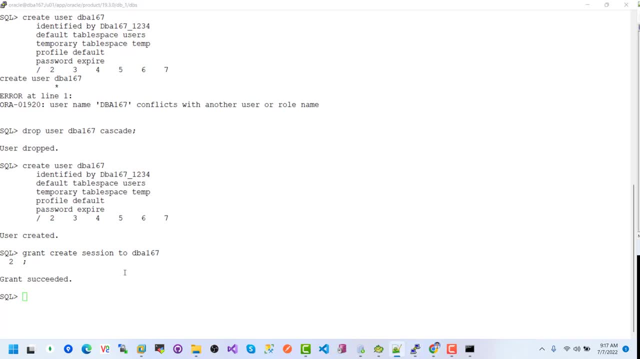 so now we will give the password exactly. uh. password for db167, future login password is star x, extension 3 or Dgpl 19503' and password value for this is Olivia's password, which is db167. underscore one, two, three, four, db167, half and under. 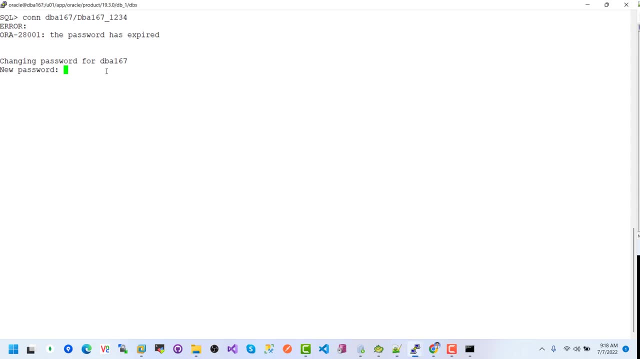 so now it ever kinda commit the password and then accept the pass, struggles ishm and then, uh, so if we connect the la contarsul a- actually I just want to give the password, he is very difficult to give the password now not bad, not, you know, not bad. so give me e underscore one six. 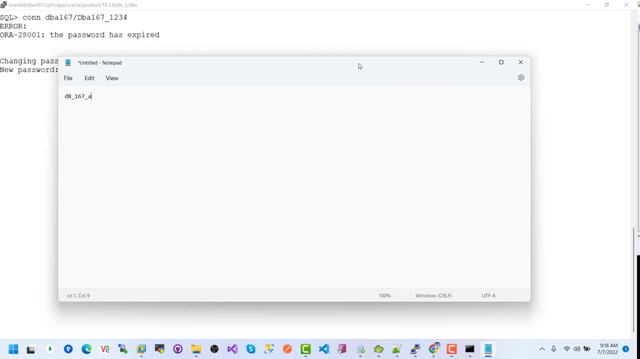 seven underscore a, b, c, underscore one, two, three underscore, so this one we will use for our password. so if I give here immediately and then password changed, so if we log in with our connect with one DBA, one, six, seven, slash. this is the newly created password, so you are no longer connected. 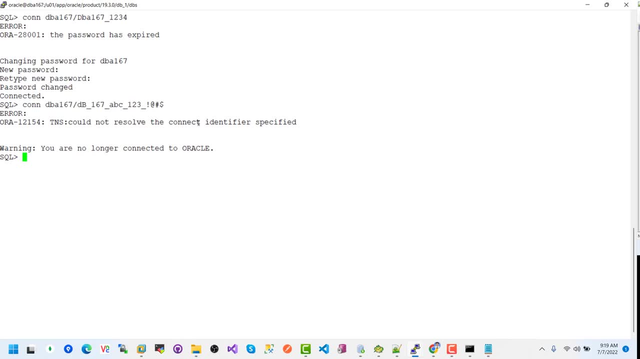 to Oracle. GNS could not resolve the connection identified specified, so there may be a problem. now I just want to change the password again. alter user: DBA one, six, seven. identified by DBA one, six, seven. underscore one, two, three, seven. underscore one, two, three, four. you can enter k, not connected. so maybe no user connected actually. so first we need to check. 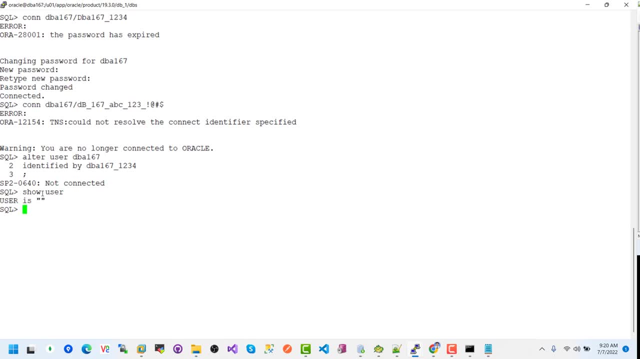 the user here. user is simply so. first we need to connect with a cc user, so phone sees this, sees one, two, three as csdba connected and if we try by using this command to connect here we can see no longer connected to oracle for user user. sorry, we need to give the password actually. 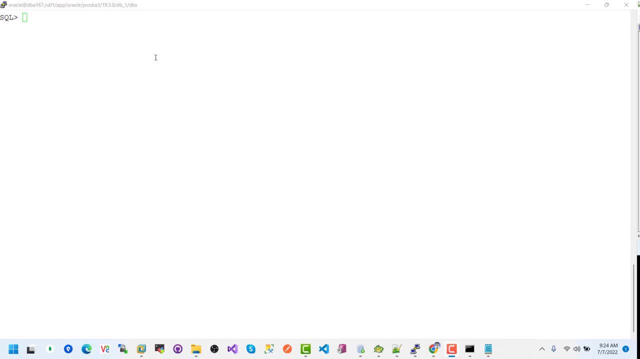 if you face these types of problems, first we need to connect with the cc directory. so on on slash as his dba, they are connected with ssdba. so alter user dba167 identified by dba167. so this is the password. uh, change comment for a user db167. so here the password db167 altered. now we will try to connect with the. 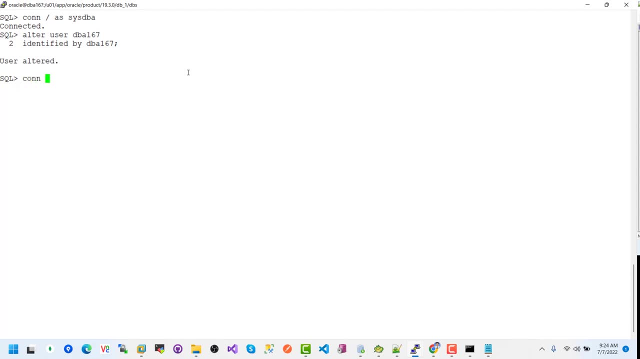 cc user, so one uh dba user x, db167 user, actually, so one dba dba167. the password is dba167. here you can see the db167 and 7 user connected. we have lots of a a system previous. let's search the google oracle list of system privileges. so 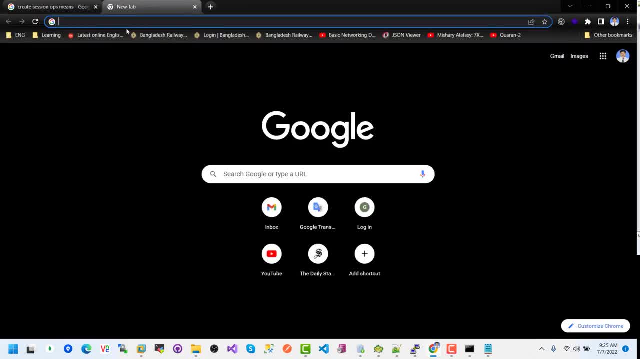 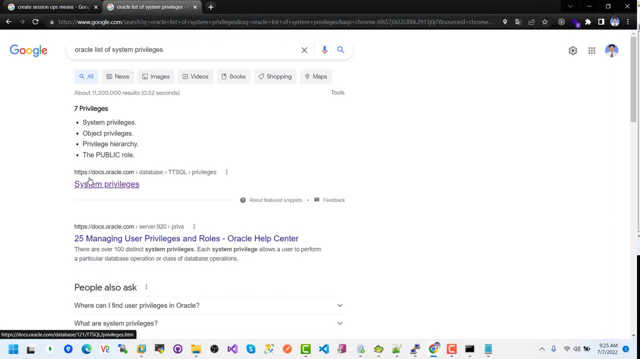 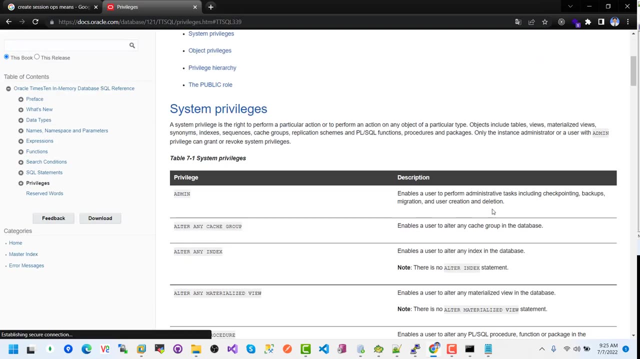 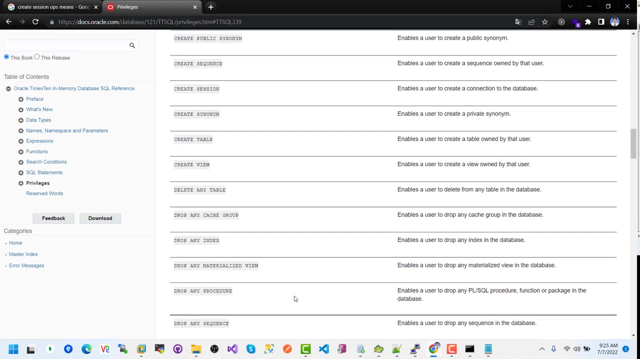 this is my um chrome browser, so i just want to search with oracle list of system privileges by hitting on enter key. we can see the first one is system privileges. just click on it. if we go down system privileges, there are lots of system privileges, so if we need to use this one, we can help from this document. 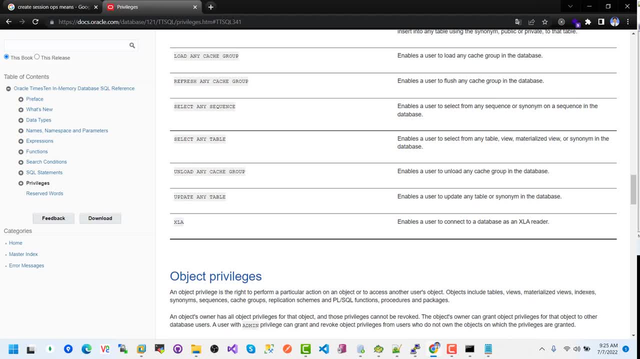 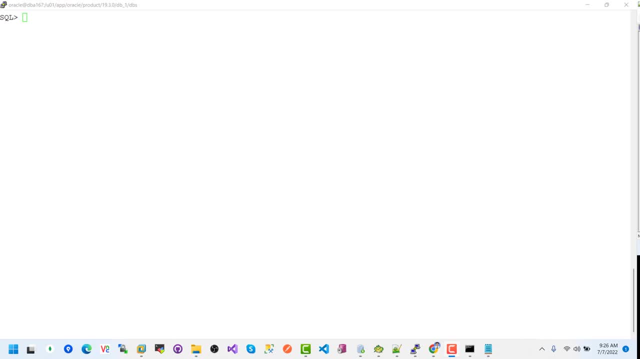 though I will give this link in description box, so don't worry about it. let's add grant privileges to create table by its own schema and other schema also. so how do you do that? first, we need to connect with sys as sysdbi. let's here grant create any table. so this is the system privilege to db167. 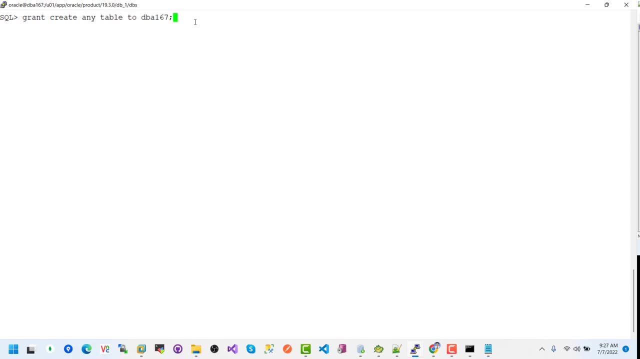 so that means this user can create its own schema table and other schema also. so after hitting enter key we can see grant succeeded and then we will give the unlimited table space permission to privilege to db167 user. grant unlimited table space to db167. now show user. 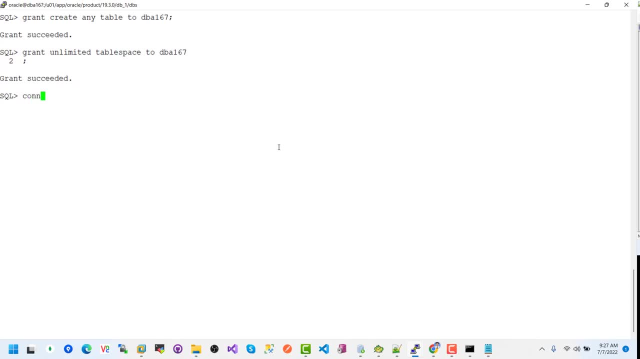 now we will create table by its own and other schema. so let's hit enter. so this is. this is the only schema table. if I hitting on enter key now, we will be able to create table created, now we will create another table with the schema name A and its. 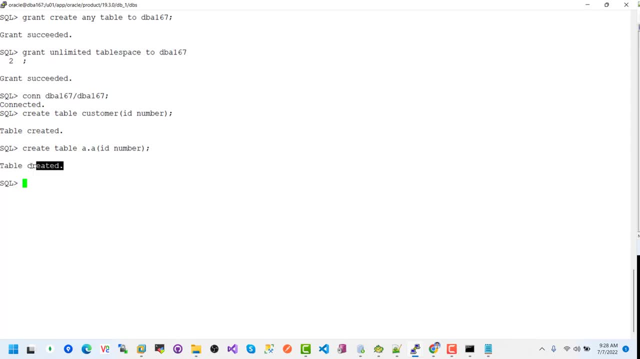 table name A actually. so if we execute this one, the command success button, let's revoke the create any table privilege. so how do you do that? evoke, create any table from DBA 1, 6, 7, revoke, create. so first we need to in insufficient privilege, that's and this: 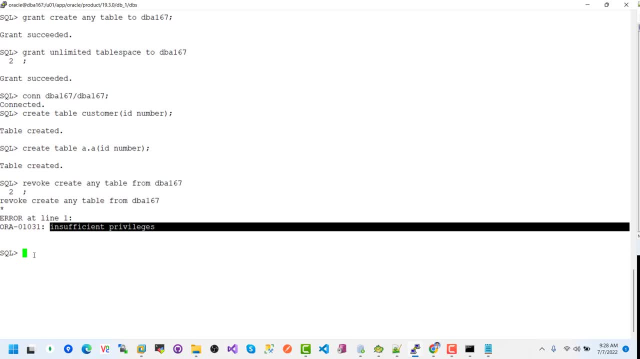 means we need to switch the user c-sexually so on. slash as cis DBA and now and execute this command again. control NPC itself. so now we can arrived here and repeat code db-1x evoking. we will pass a command right now. here we have here: db-1x revoked successful. 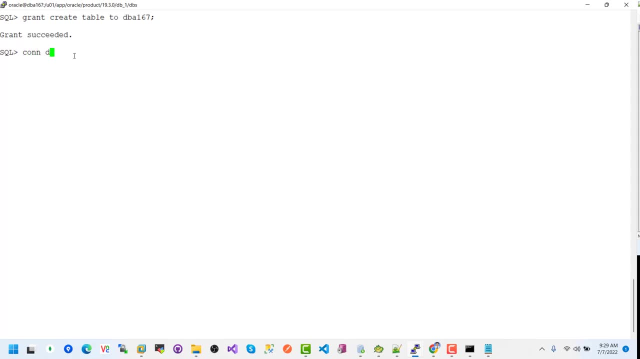 revoked successful DBA 167, slash DBA 167 CR and now try to do create a table to schema A and it will return an error. so let's try create table. this is the A schema and the table themselves. so after hitting an interkey we see insufficient privilege. so in this way the system privilege work on. 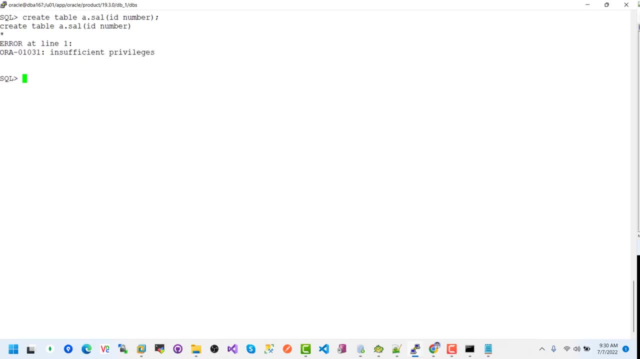 a specific user. so hope you guys enjoyed this tutorial. don't forget to subscribe my channel. keep watching the next tutorial. thanks.